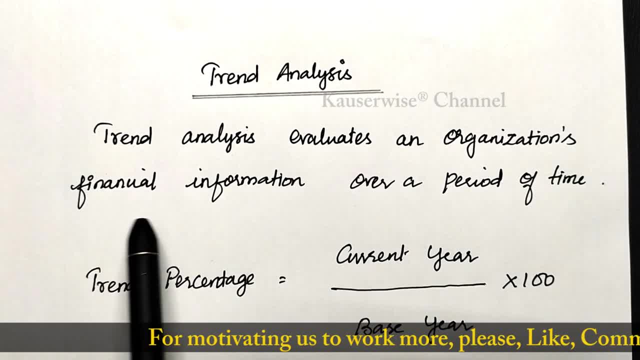 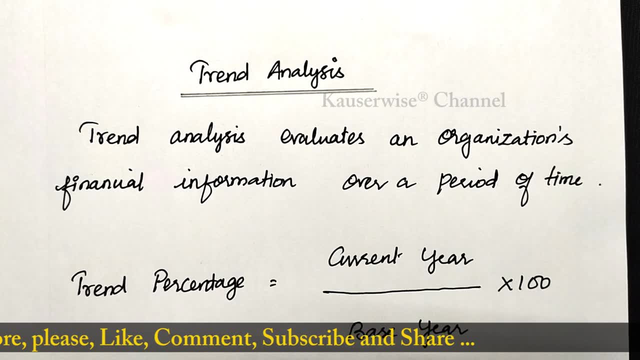 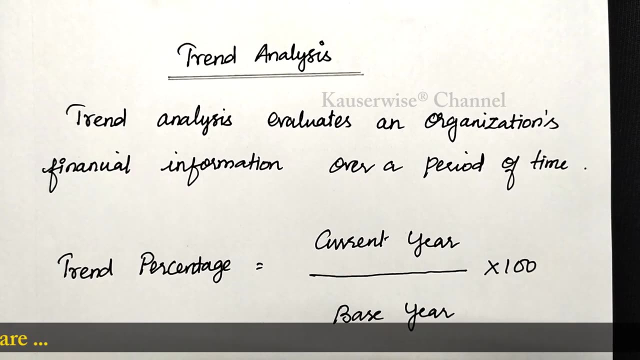 Trend analysis evaluates an organization's financial information over a period of time. So often it is used to evaluate each line of items on the income statement as well as balance sheet. There is a formula to find out trend percentage. The formula is current year data divided by base year data into 100.. 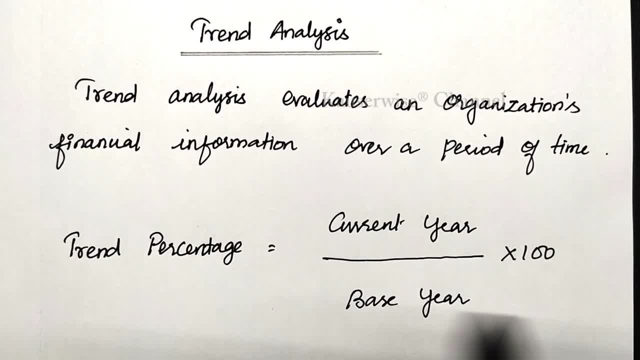 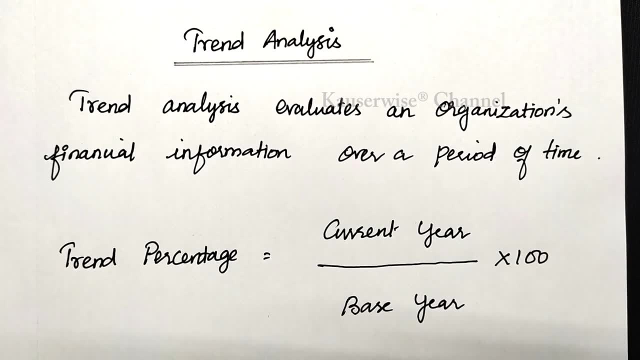 So this percentage, that is, 10%, This trend percentage is applicable for each and every item of income statement, as well as balance sheet information. Now we will see one numerical problem. to have a better understanding of trend analysis, Look at the problem. 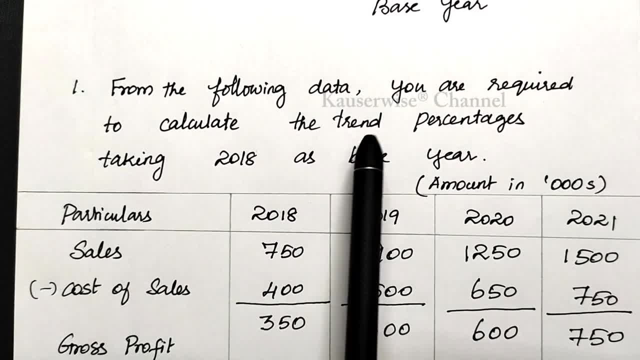 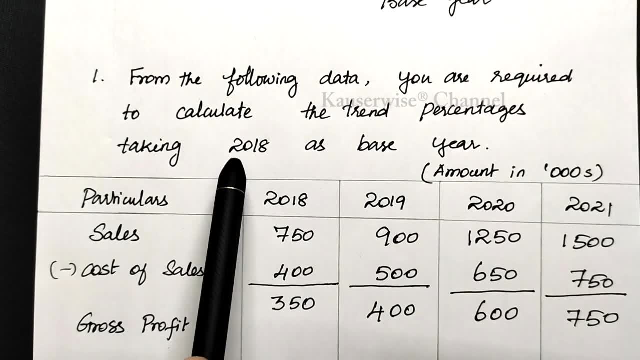 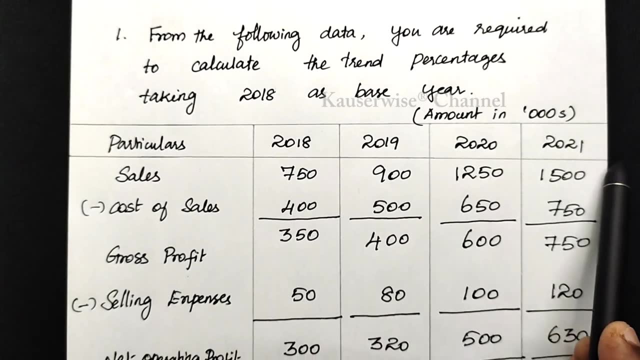 From the following data you are required to calculate the trend percentages, taking 2018 as base year. So here they have clearly mentioned that 2018 data is the base information. Based on that we are going to calculate trend percentages. So in this case, we will calculate trend percentages, taking 2021 as base year. 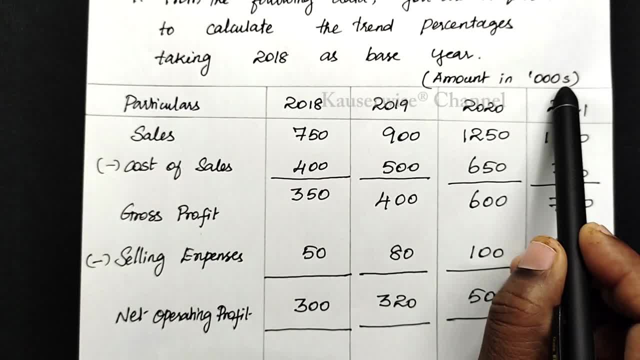 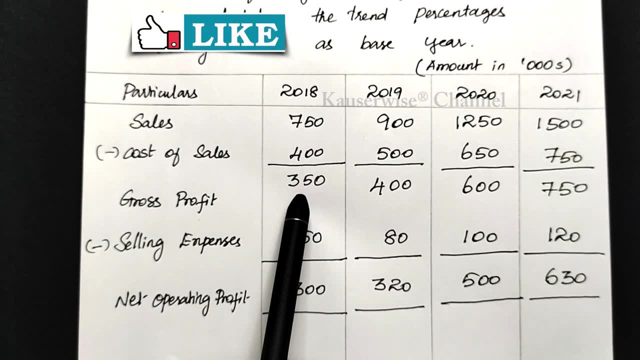 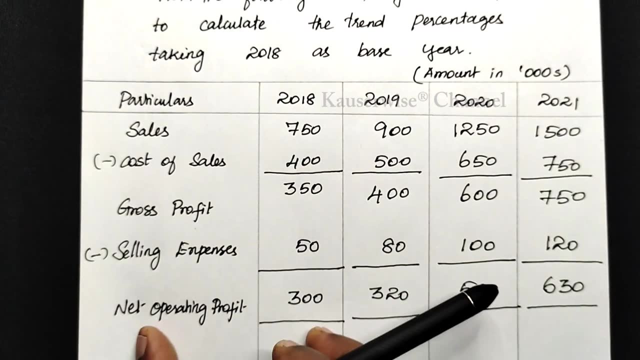 But before that, let us see the scenario where we see that trend and value are completely opposite. Instead, we will take a look at the previous data. So here we have seen that the trend percentage taking 2019 as base year and the value taken as base year. 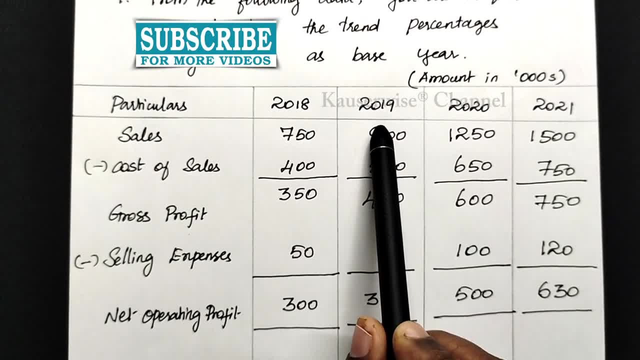 If you take the trend, you will find that the trend percentage taking 2019 as base year is less than 0.5%. The trend percentage taking 2020 as base year is less than 0.5%. Now let us predict the trend percentage. 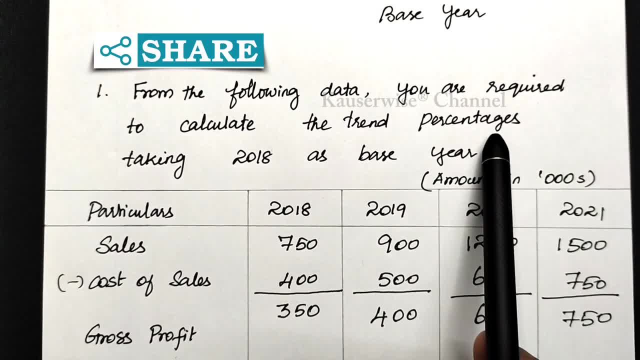 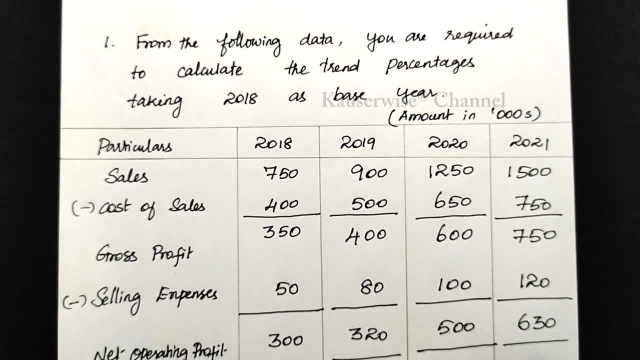 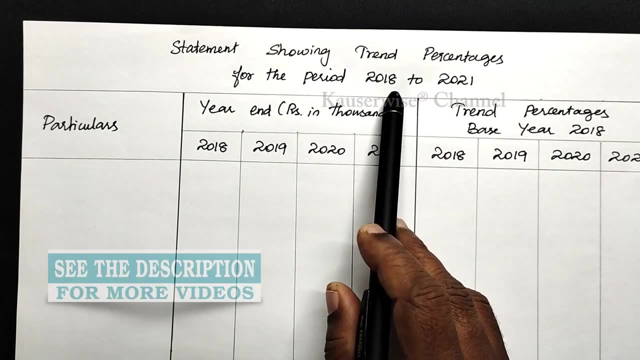 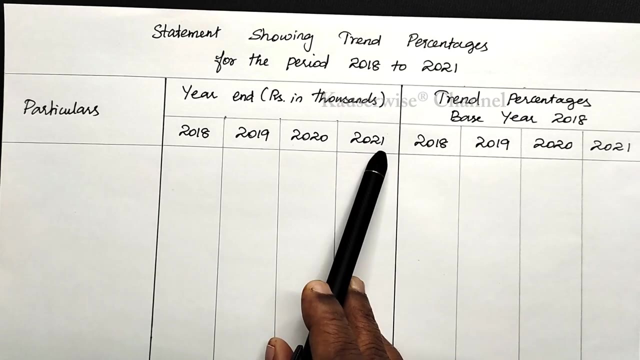 Here we have given all the values, Amounts in thousands. they ask you to prepare trend percentages, taking 2018 as base year. Now let us see the solution to prepare trend percentages. Look at the solution table statement showing trend percentages for the period 2018 to 2021. particulars: year end: at the end of 2018, 19,, 20,, 21, all the datas, that is. 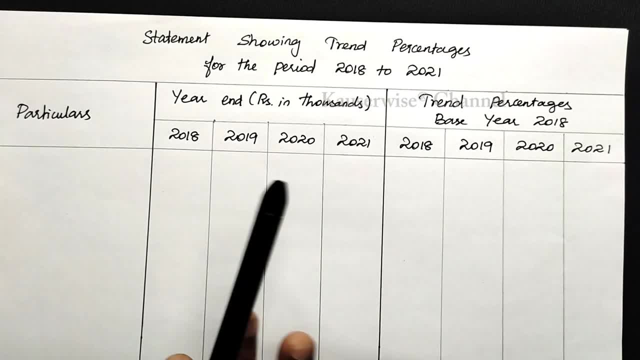 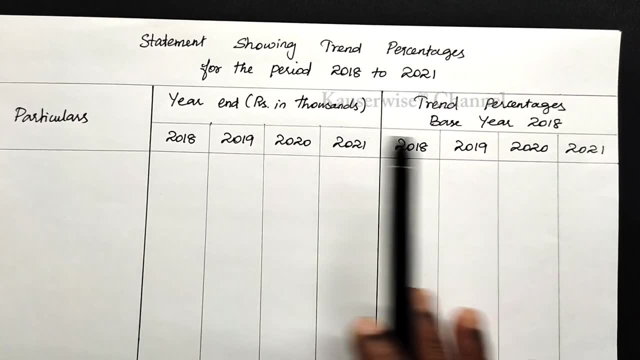 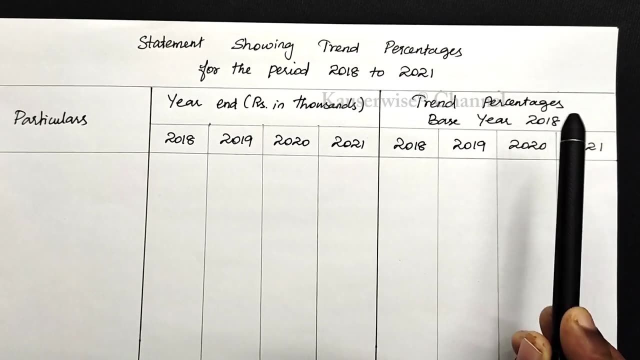 rupees in thousands. So that is given in the problem know. we are going to record the particulars and the data from the question as it is. After recording all the information, we are going to calculate trend percentages. base year is 2018.. So this information is given in the problem know. 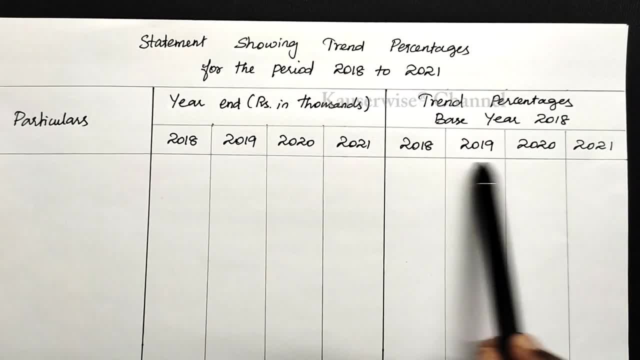 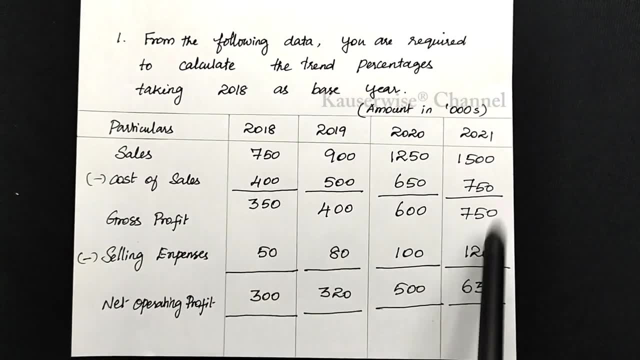 based on that, we are going to calculate trend percentage for all the other years. Now let us see the question. Look at the question. just copy the particulars and amount for 2018,, 19,, 20,, 21- all the data from the question as it is. After recording all the information, we are. 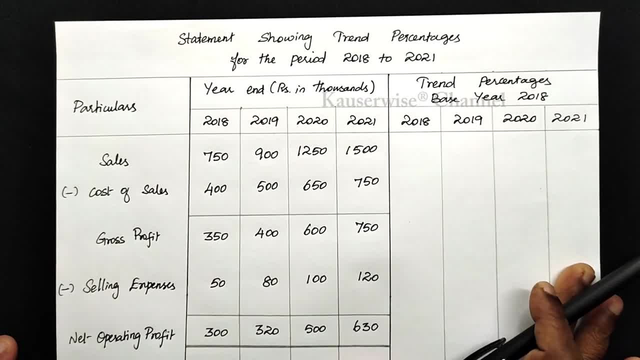 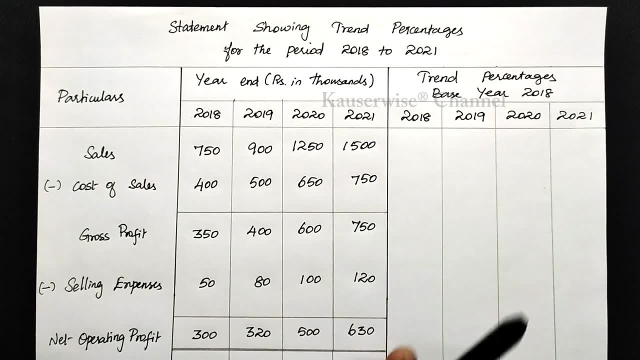 19, 20, 21 in the solution table- See the solution. I have entered particulars and years. that is, amount for 2018, 19, 20, 21. from the problem as it is. With this information we are going to calculate. 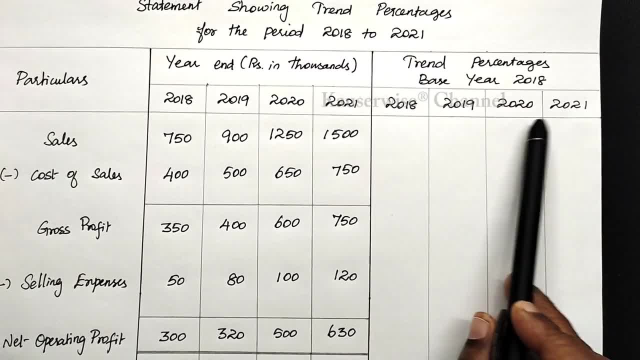 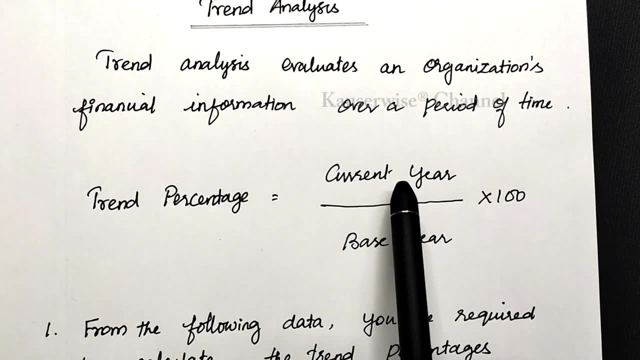 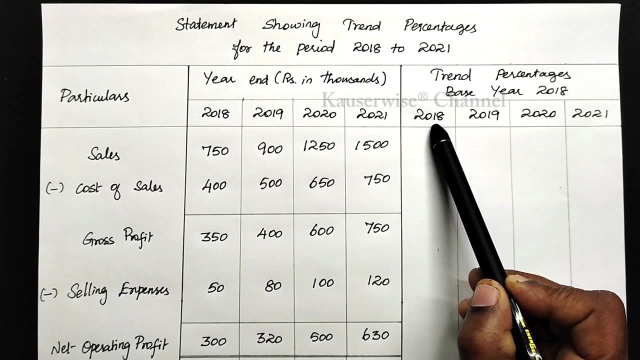 trend percentages for 2018, 19,, 20, 21.. What is the formula for trend percentages? Look at the formula. trend percentage is equal to current year divided by base year into 100.. See the solution for 2018. we are going to get 100 percentage for each and every item. The reason is: 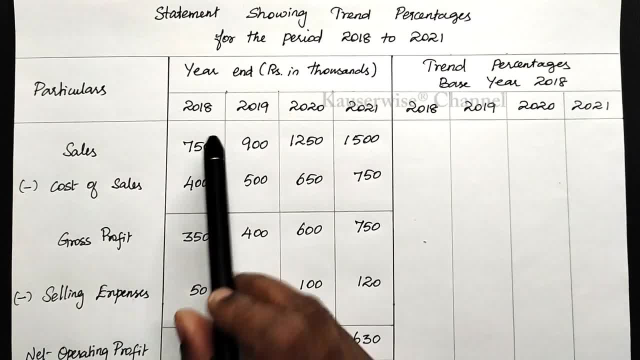 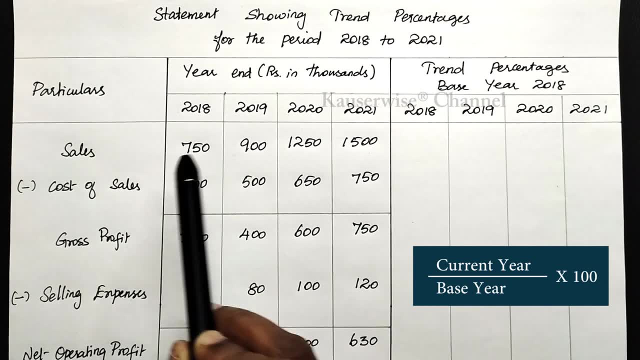 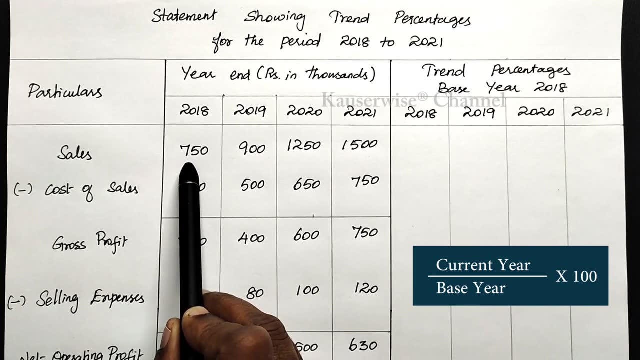 2018 is the base year. Just see the first one sales 750.. What is the formula? Current year data divided by base year into 100.. So current year is for 2018. I am telling 750 divided by base year. same thing 2018: 750 into 100.. So 750 by 750 into. 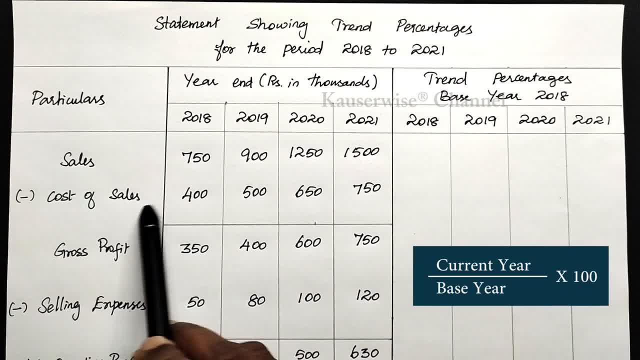 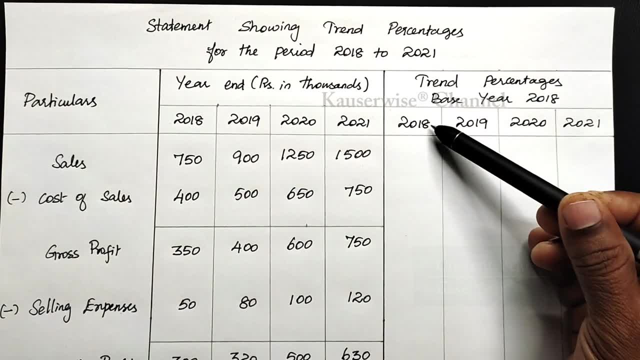 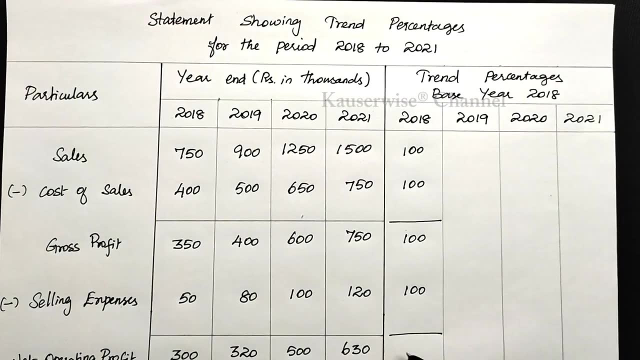 100, you will be getting 100 percentage. In the same way, the next item: 400 by 400, 1.. 1 into 100: 100.. So for 2018, we will be getting 100 for each and every item. Okay, in the same way, we need to. 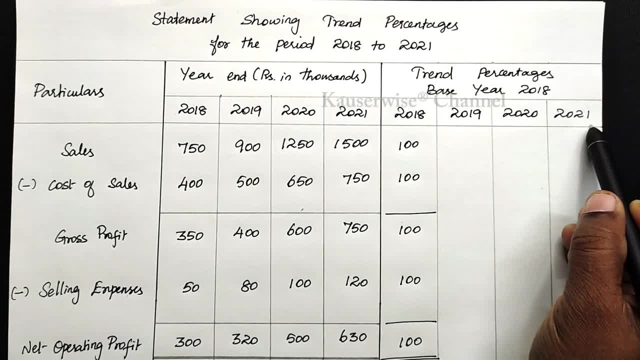 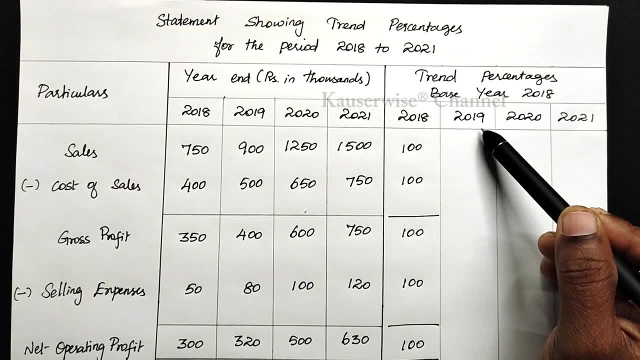 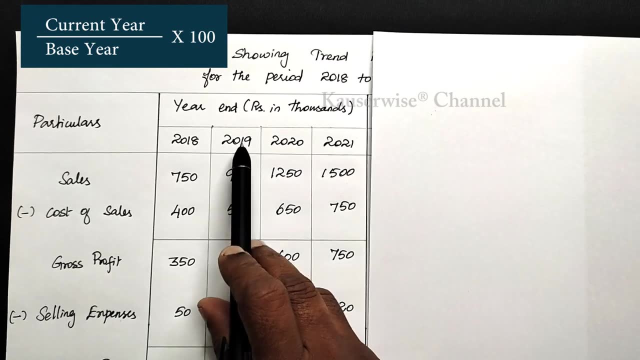 calculate trend percentage for 2019, 20, 21.. If we get any decimal, you can round up the figure. Simply apply the formula. Now let us see the calculation for 2019.. So what is the formula? Current year data divided by base year data into 100.. So for 2019, the first information is sales. 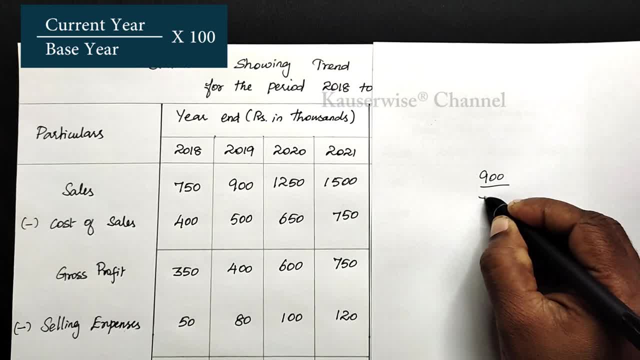 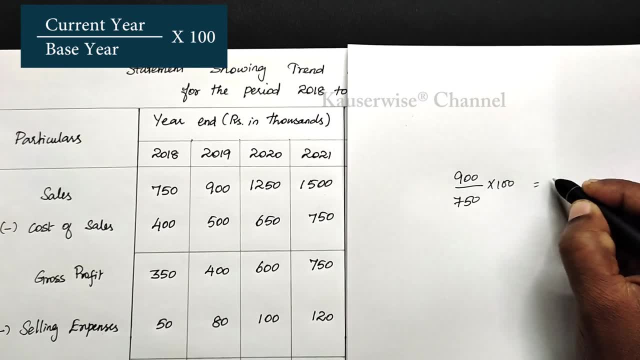 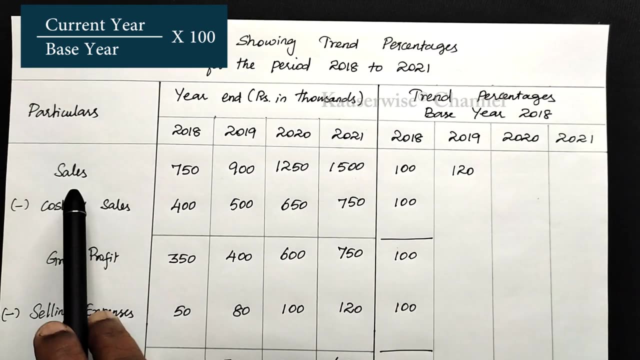 no, 900.. 900 divided by 750.. Base year is 2018. information: 750 into 100.. So what is answer? 120.. So 120 percentage: See the trend percentage for 2019.. That is the first information sales. How much percentage? 120 percentage, Okay, In the same way. 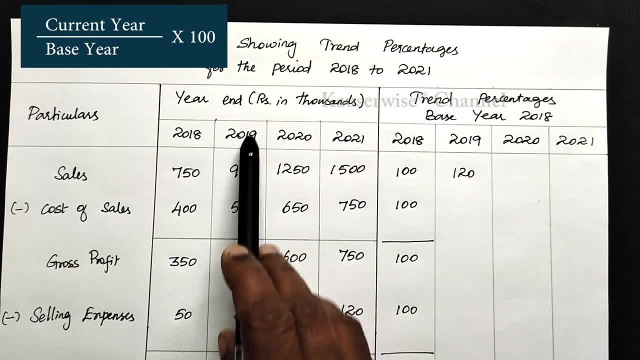 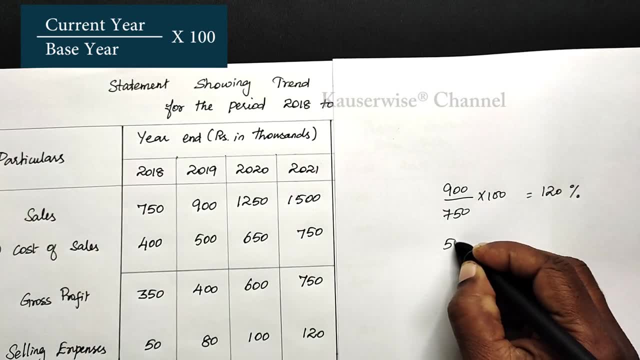 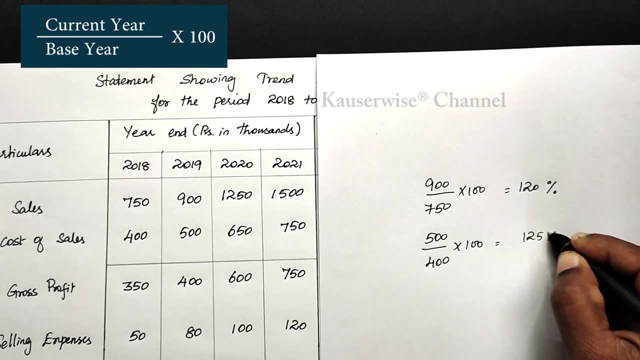 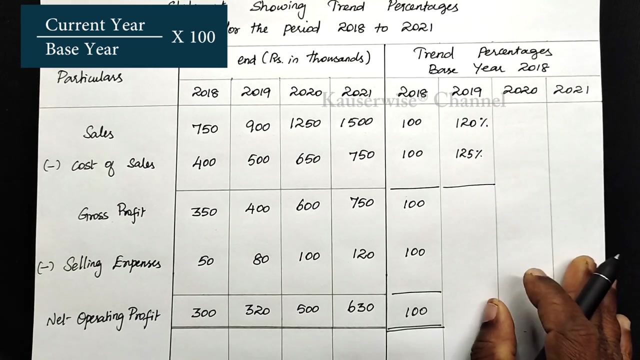 calculate. for other information, The next one: cost of sales For current year 500 divided by base year, 400 into 100. Answer: 125 percentage. So enter 125 percentage. In the same way, we need to calculate trend percentage for each and every individual item. Okay, for 2019. the next information is GP. 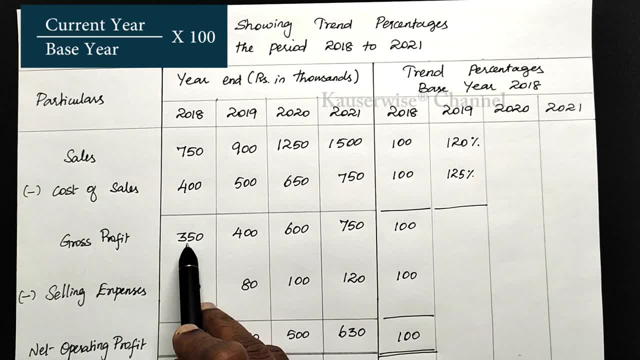 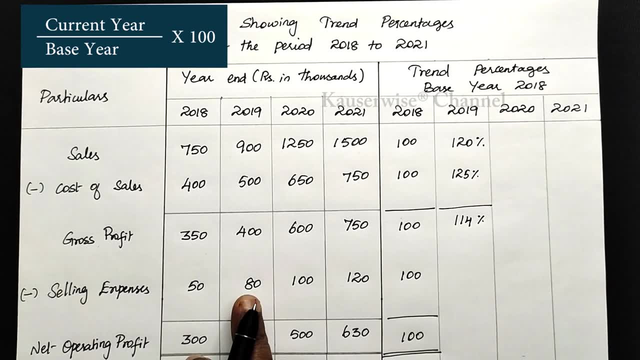 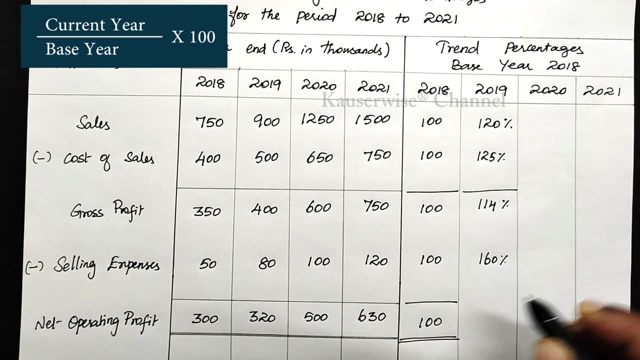 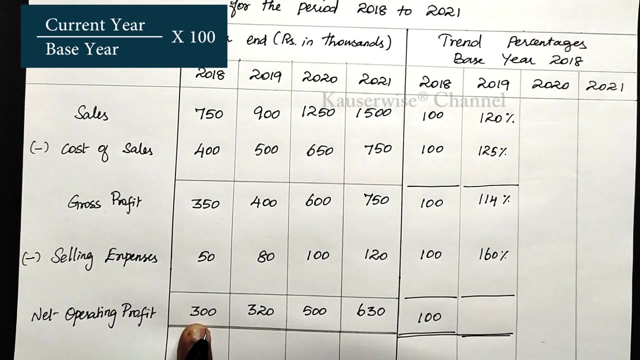 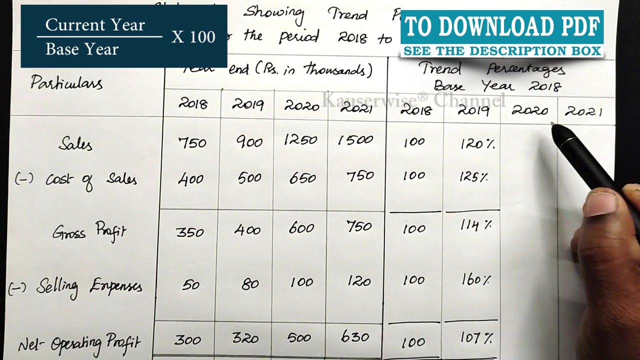 Gross profit: 400 divided by 350 into 100. 114 percentage. The next information selling expense: 80 divided by 50 into 100. 160 percentage. Then the net operating profit: 320 divided by 150.. So 300 into 100. 107 percentage. Okay, in the same way we are going to calculate trend percentage for. 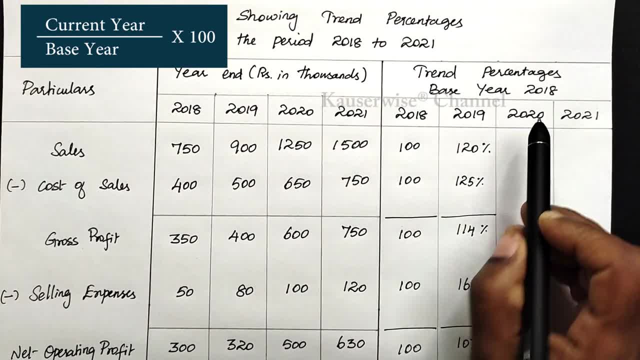 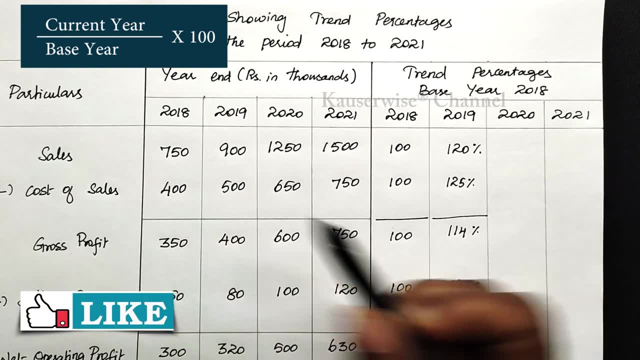 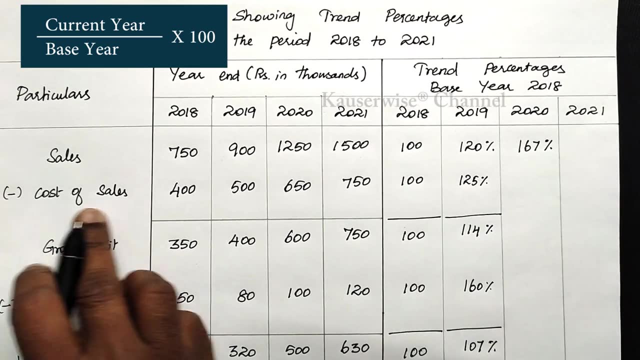 2020 as well as 2021.. For 2020: 1250 divided by base year: same 2018.. 750 into 100.. 167.. You have to round up the figure, Okay, and then the next item: cost of sales for 2020.. 650 divided by base. 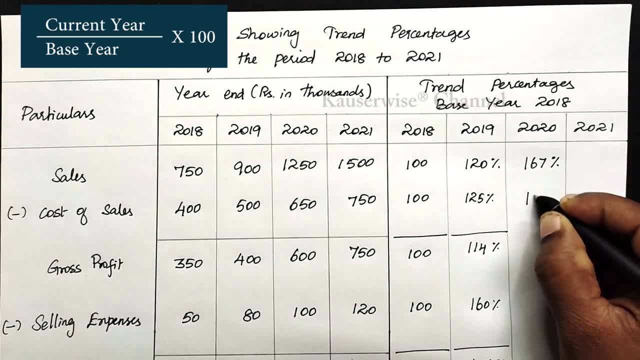 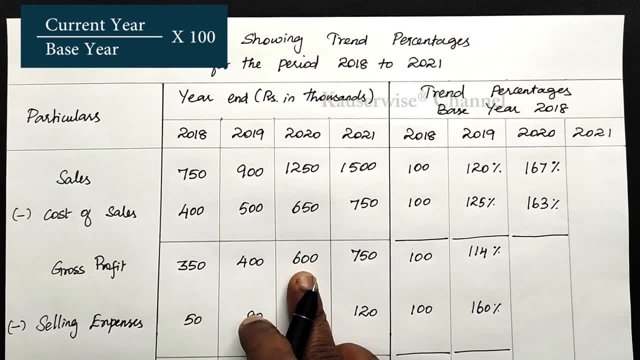 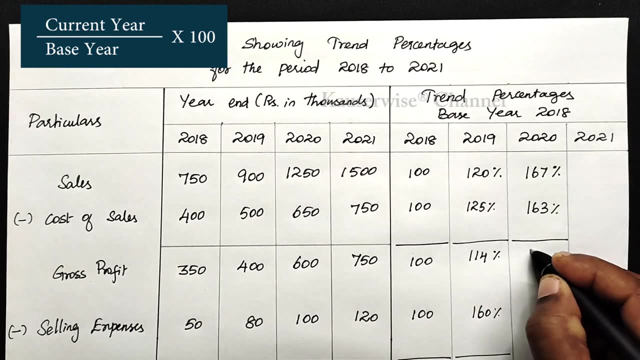 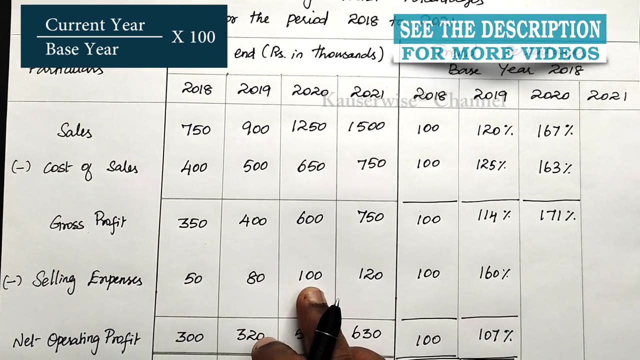 year. 400 into 100.. 163 percentage. Then gross profit for 2020.. 600 divided by base year is 2018.. No, 350 into 100.. 171 percentage. The next one selling expense for 2020.. 100 divided by 50 into 100.. 200 percentage. 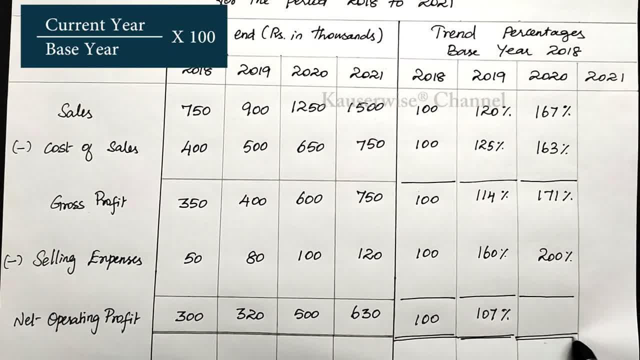 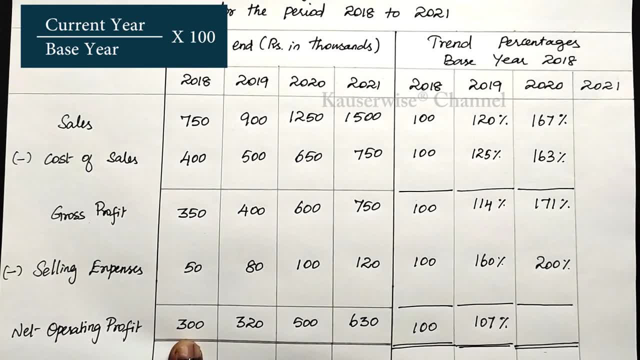 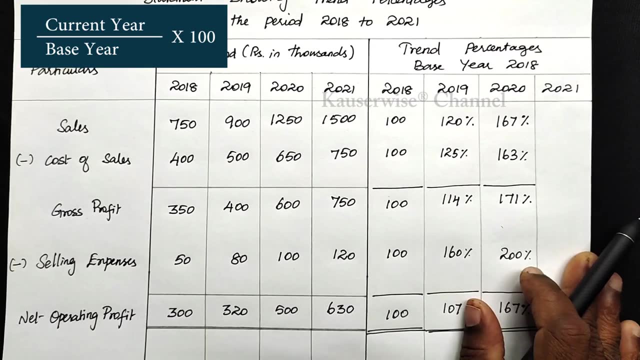 Okay, so now net operating profit for 2020: how much? 500.. So 500 divided by base year, 300 into 100.. 167 percentage. Now calculate percentage for 2021.. So 2021 is the current year. no, So current year.